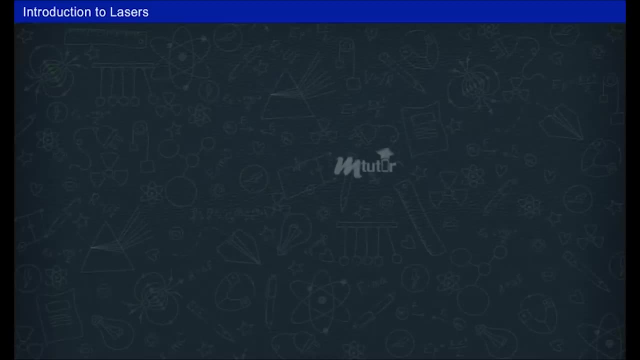 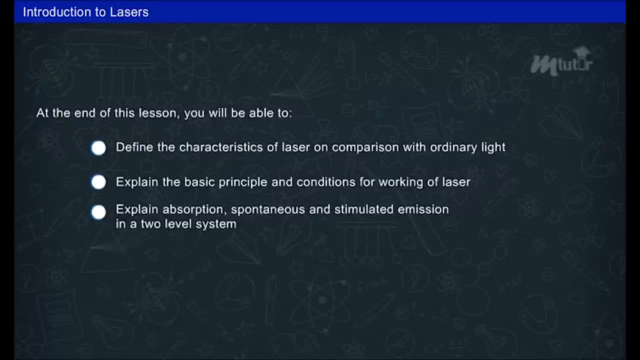 Introduction to lasers. At the end of this lesson, you will be able to define the characteristics of laser on comparison with ordinary light. explain the basic principle and conditions for working of laser. explain absorption, spontaneous and stimulated emission in a two-level system. list the properties of laser. 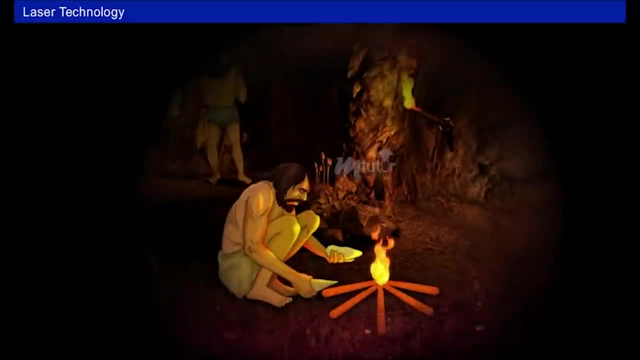 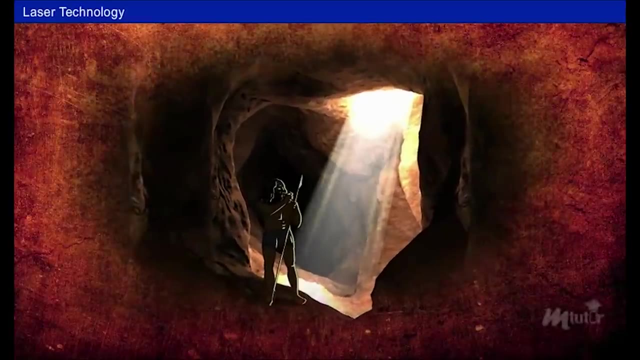 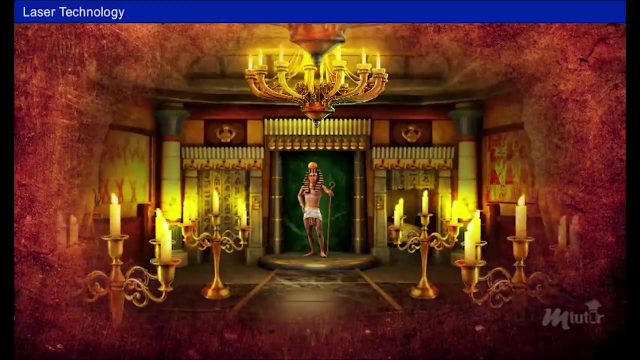 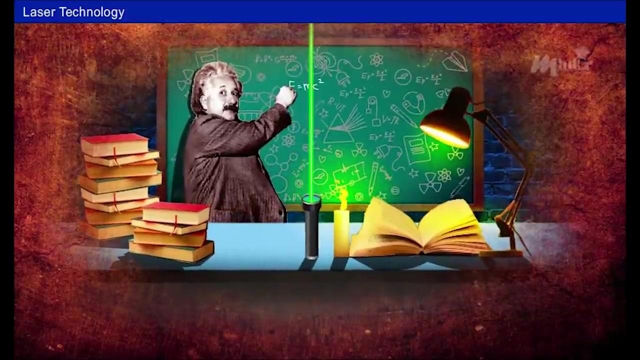 and the basic principle of light. The fear for darkness vanished when man discovered fire. Till then, man knew only the natural sources of light. Later, light source evolved into different artificial forms. Physicists had worked to create devices for producing powerful beam of light. 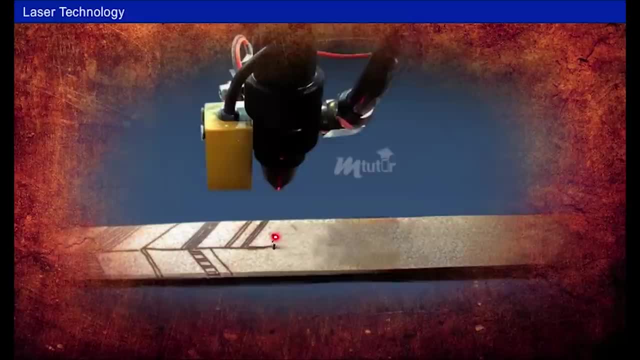 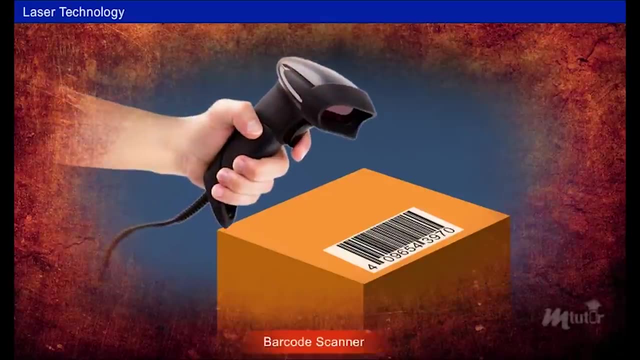 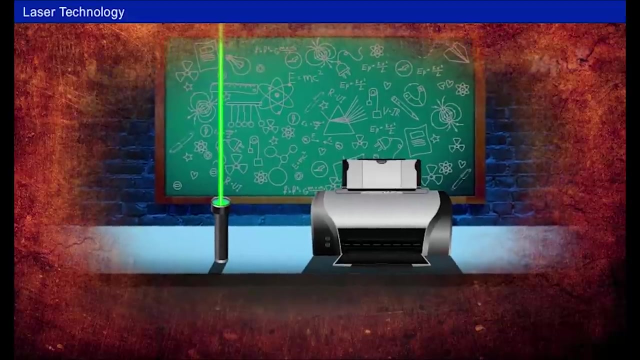 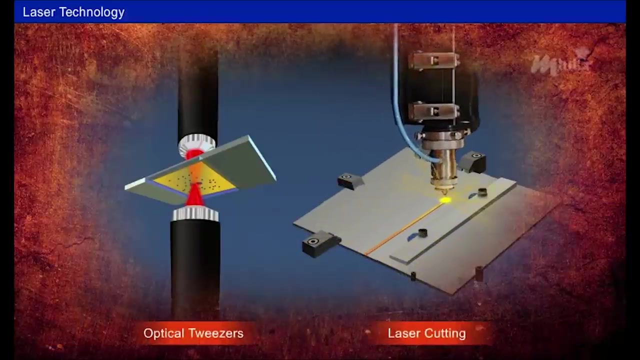 This resulted in the invention of lasers. Lasers are an important milestone in the field of engineering, in science: From a barcode scanner to intruder detection in high-security areas. From a projection pointer to printers. From optical tweezers for handling delicate matter to cutting off high-strength materials. 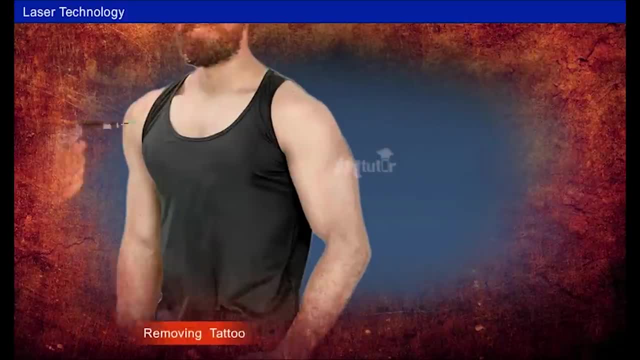 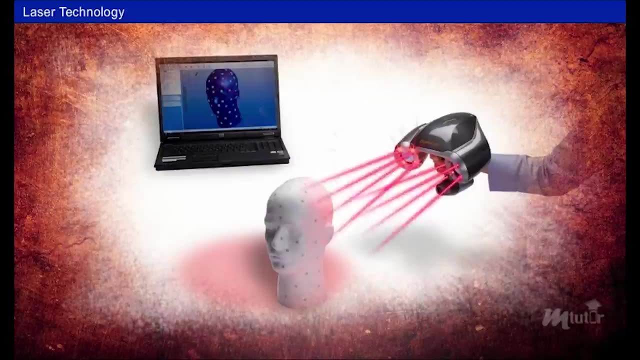 From a laser pointer to a laser printer, From a laser pointer to a laser printer, From removing body art to complicated eye surgery, Lasers are simply everywhere. Lasers have unique characteristics differing from ordinary light. This enables to produce highly intense light focused to a small point. 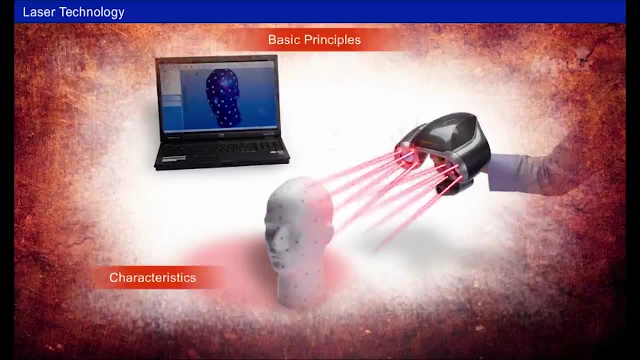 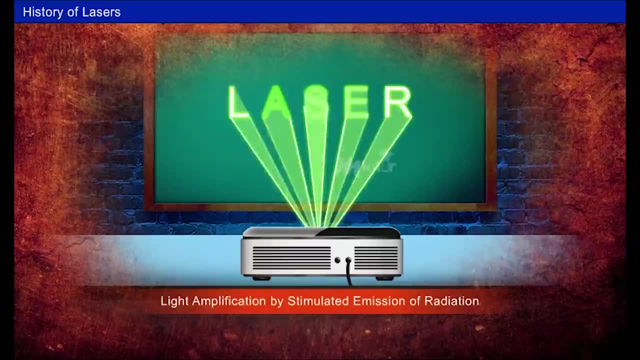 Next, let us discuss the basic principles, characteristics and working of a laser. The term laser is an acronym of light amplification by stimulated emission of radiation. The term laser is an acronym of light amplification by stimulated emission of radiation. It is a device which produces an intense beam of monochromatic and coherent light. 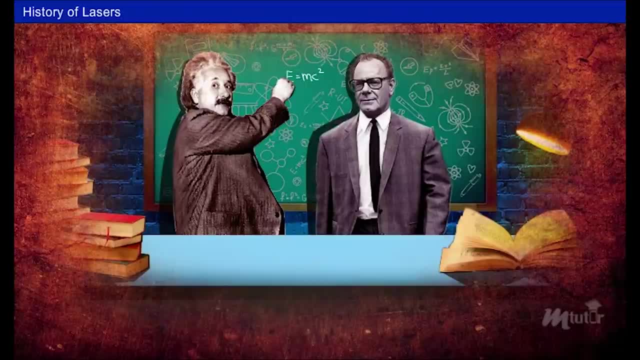 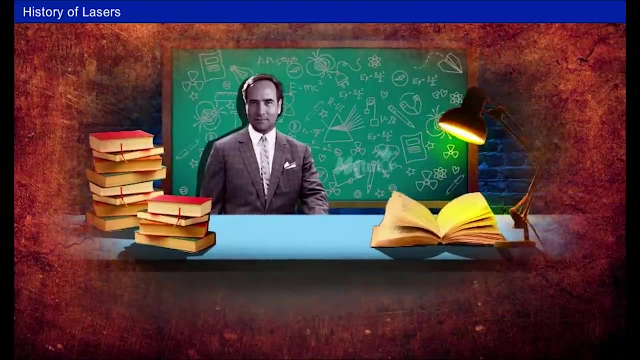 Every invention has some history, So indeed lasers. The basic principle of laser is based on the Einstein's theory of light, proposed in 1916, which was later developed by Gordon Gould in 1957.. In 1960, Theodore May Mann invented the first working ruby laser. 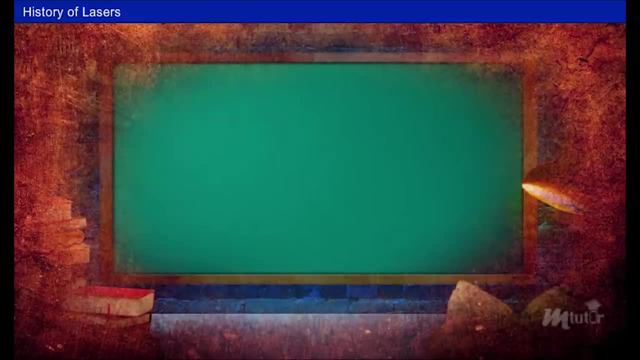 which was also the first optical laser. Apart from solids such as ruby, researchers have analyzed that some materials like xenon, helium or semiconductors can also be used as laser mediums. Different types of lasers have been developed, which enhanced the scope of their applications. 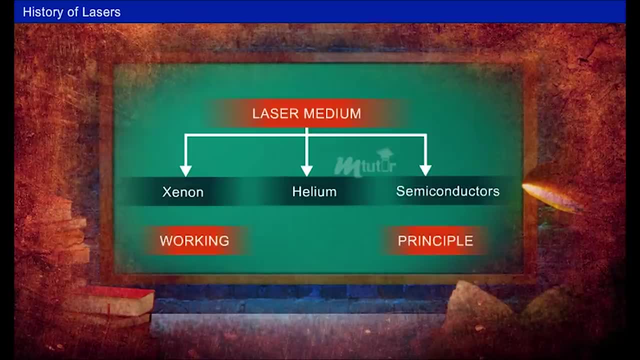 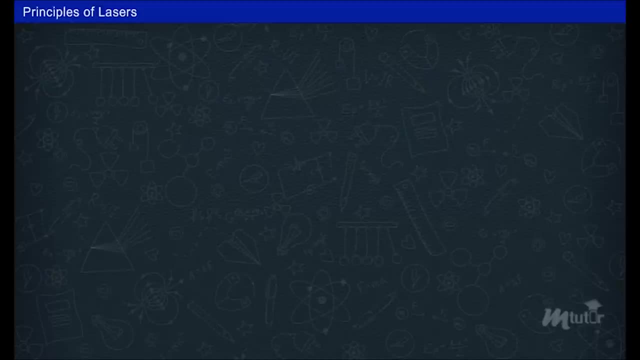 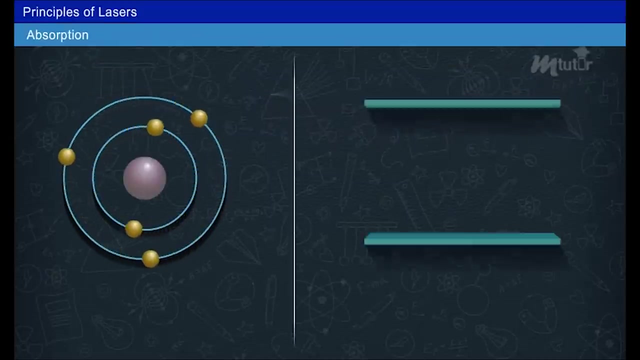 The working and principle of the laser is based on some important features. Let us discuss about them. The working principle of lasers is based on spontaneous absorption, spontaneous emission, stimulated emission and population inversion Absorption: An atom consists of different energy states. Let us consider two different states of an electron. 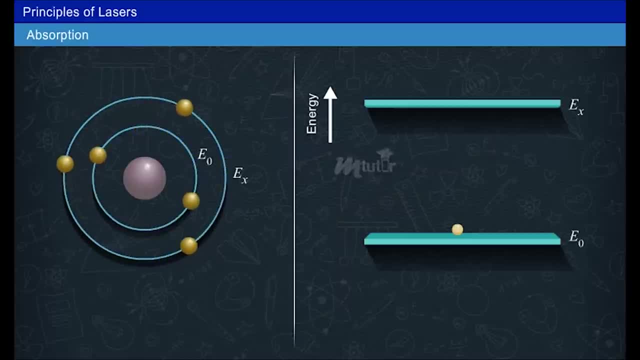 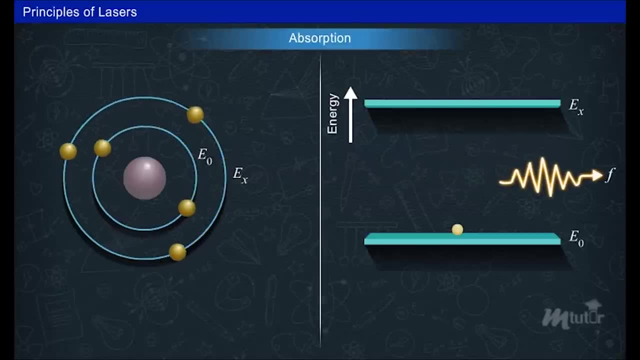 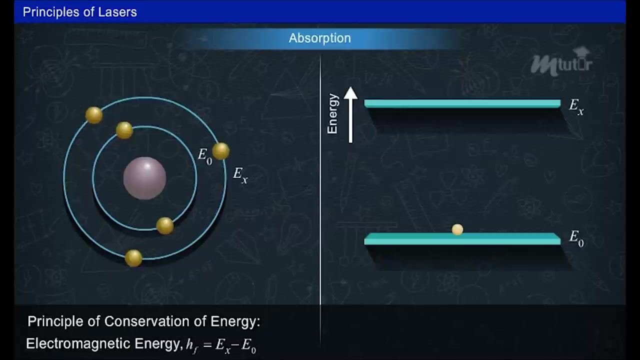 such as ground state E0 and excited state Ex. Electromagnetic energy falls on an atom in the form of photon of frequency F. From the principle of conservation of energy, the electromagnetic energy is given as the difference of Ex and E0. When the photon energy falls on the electron, 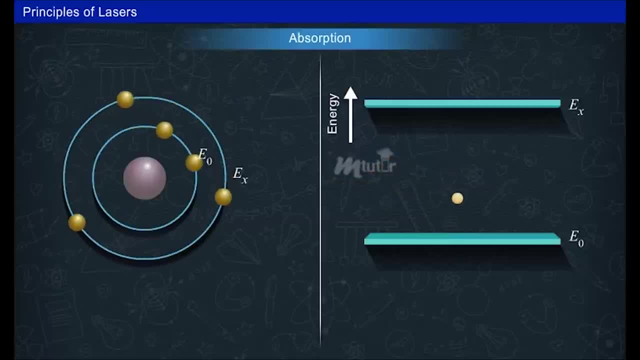 it jumps from the ground E0 to the excited state Ex by absorbing the energy. This process of absorbing energy from photons is known as absorption of radiation- Spontaneous emission. It is known that electron absorbs energy and moves from lower energy level E0 to the higher energy level Ex. 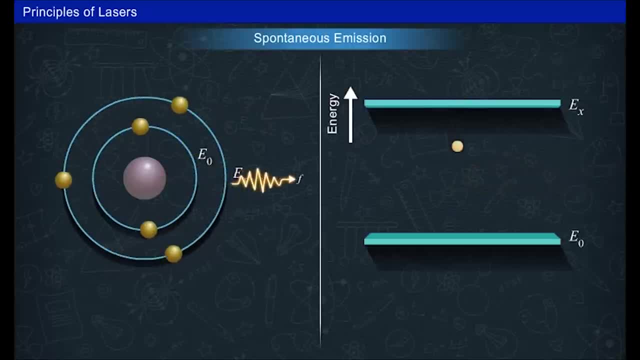 But the excited electrons that had jumped to the higher energy state does not remain in the same state for a long period and comes back to its original ground state, E0, by losing its energy in the form of photons. These photons are considered as incoherent light. 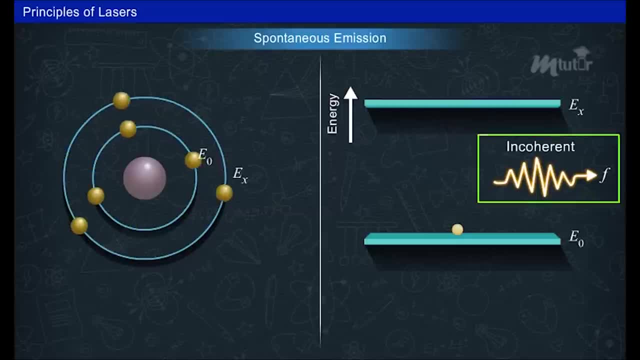 as they do have any correlation in phase. Thus the electrons in the excited atoms are released on their own from their higher energy state to the ground state, emitting photons. This is called as spontaneous emission. The mean life, or lifetime, of the excited atom is the time for which it stays in that state. 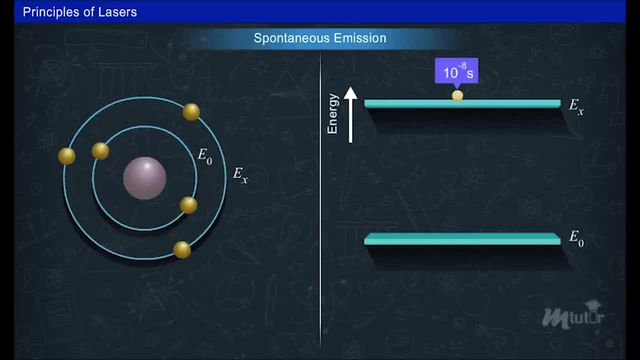 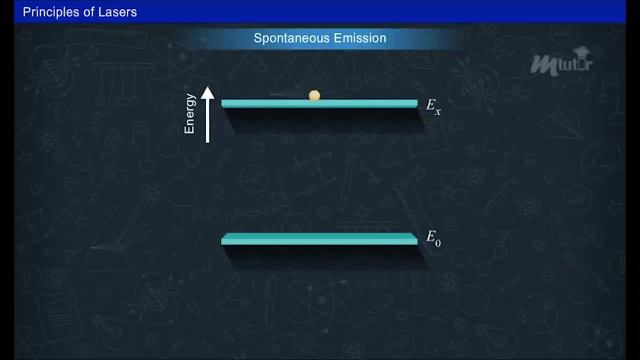 This is about 10 to the power minus 8 seconds before spontaneous emission. However, the mean life for some excited states is 10 to the power- 5 times longer, and such states are called as metastable state and they play an important role in laser operation. 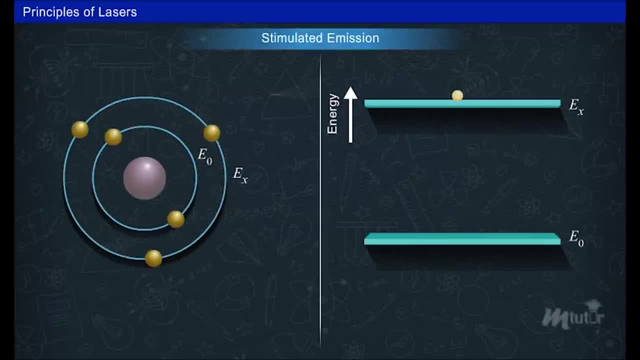 Stimulated emission. In this process, the atom is initially present in its excited state Ex. A photon of energy HF can stimulate the atom to move to its ground state E0.. During this process, the atom emits an additional photon with the same energy HF. 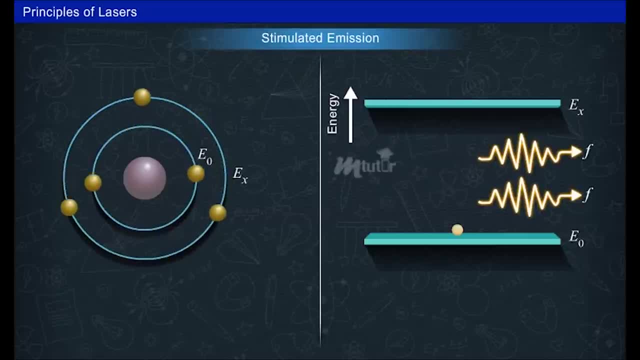 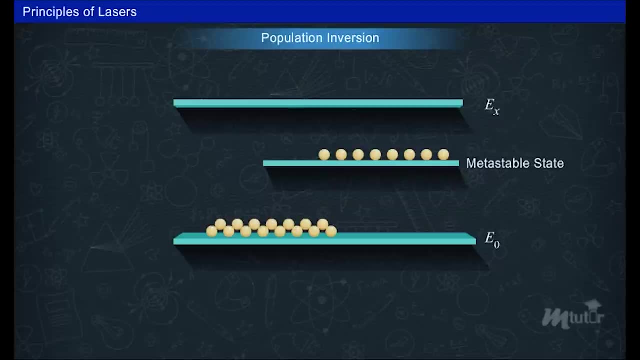 This process is called as stimulated emission, as it is triggered by an external photon Population Inversion. Generally, in any atomic system, the number of atoms in the ground state is more than that in the excited state. This is because of the tendency of electrons. 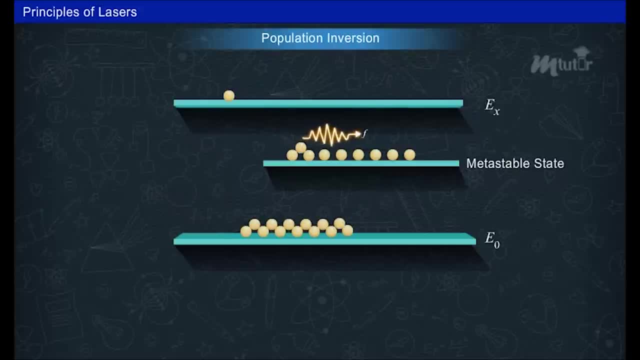 to stay in the ground state, But in order for more photons to be emitted, there should be more electrons in the excited state. This process is achieved through optical pumping, and this occurrence is known as population inversion. The transition electrons do not stay in an excited state. 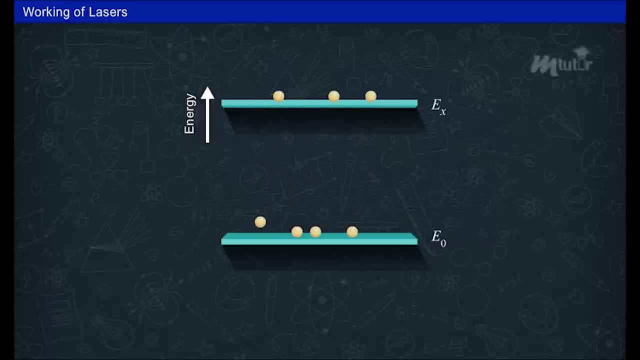 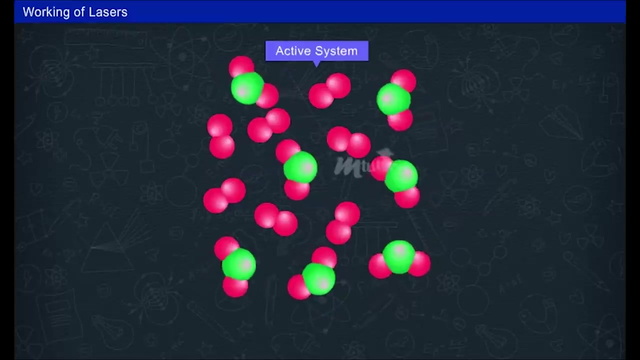 for a longer time. But in some systems the electrons remain in an excited state for a longer period. These systems are called as active systems or media. Generally, these active systems are compounds or mixtures of different elements. Consider the active system containing a large number of atoms. 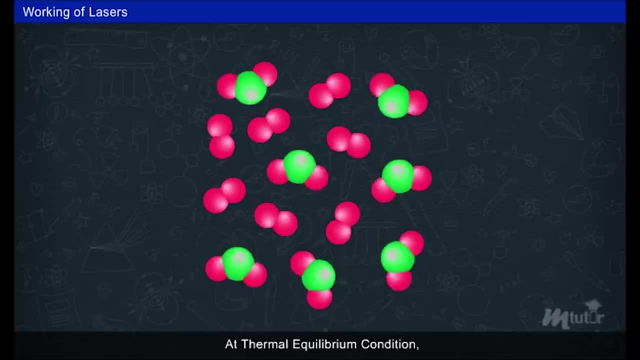 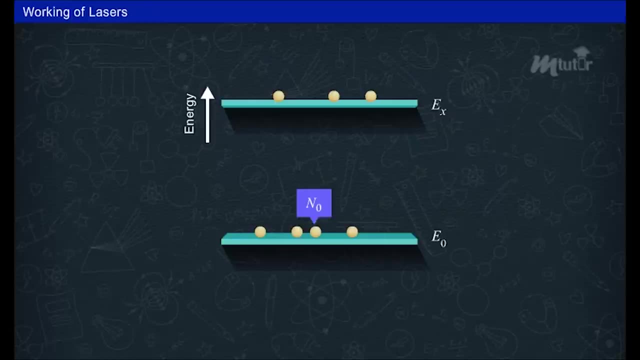 in thermal equilibrium condition at a temperature T Before the system is subjected to any radiation. there are N0 number of atoms present in their ground state with energy E0 and a number Nx are in a state of higher energy Ex According to Ludwig Boltzmann. 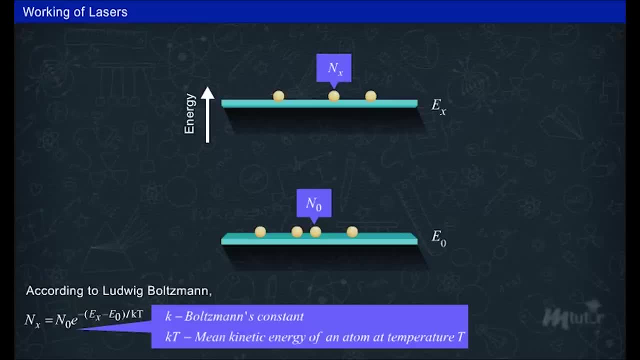 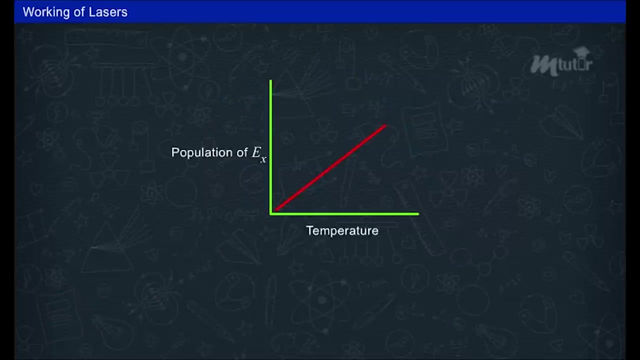 Nx can be given in terms of N0.. Nx is equal to N0 into e, to the power of minus of Ex, minus E0 divided by kT. As the temperature increases due to thermal agitation, more number of atoms move to the higher energy state, Ex. 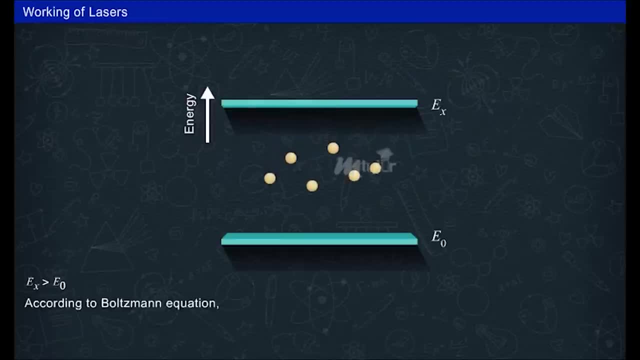 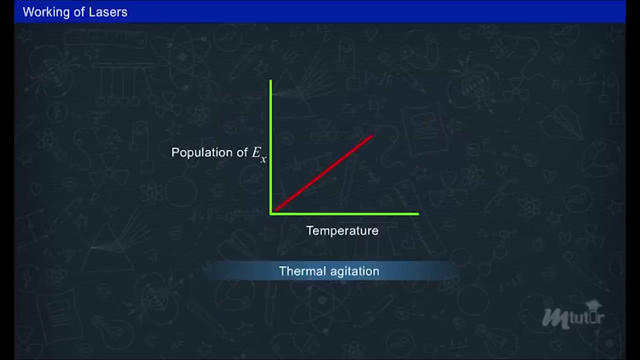 Since Ex is greater than E0, the Boltzmann equation requires Nx to be lesser than N0, means there will be less number of atoms in the excited state compared to the ground state. Thus, only by thermal agitation the populations of Ex can exceed that of E0. 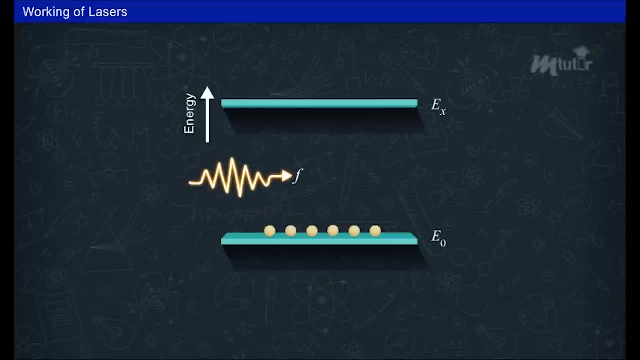 Suppose the atoms are flooded with the photons of energy Ex minus E0. Then, by absorption by ground state atoms, the photons will disappear and atoms move to excited state, leading to population inversion. Thus, through stimulated emission of excited state atoms, more number of photons will be generated. 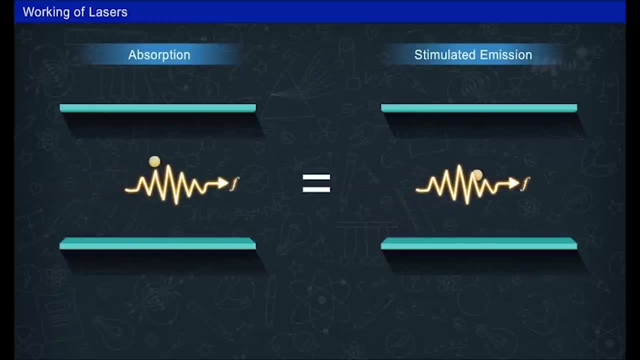 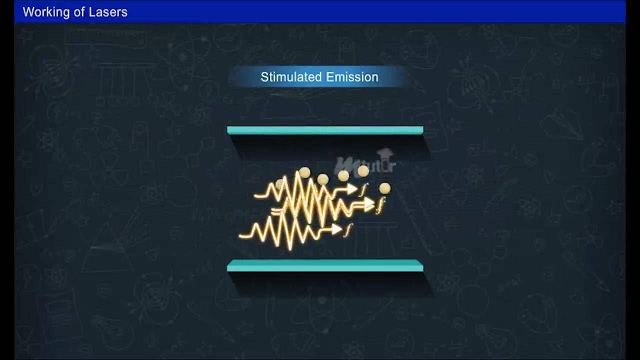 Einstein showed that the probabilities per atom for absorption and stimulated emission processes are identical. Thus the net effect will be absorption of photons when more atoms are in the ground state, When stimulated emission dominates, that is, when more photons are emitted than the absorbed photons. 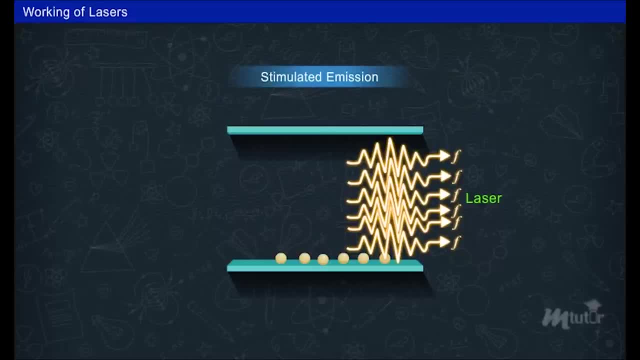 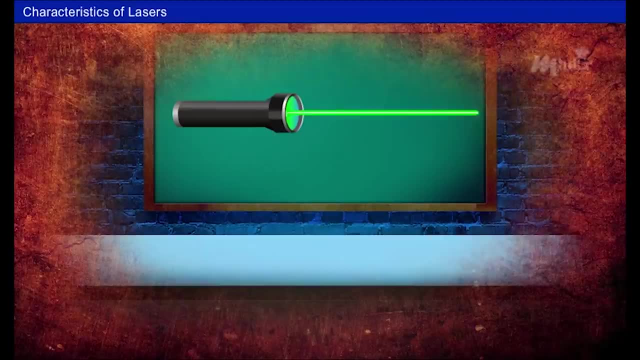 the laser light is produced. The lasers have certain unique characteristics that enable the laser light to be focused hundred times better than the ordinary light. These characteristics are monochromaticity, coherence, directionality and sharp focus. Let us discuss these in detail. 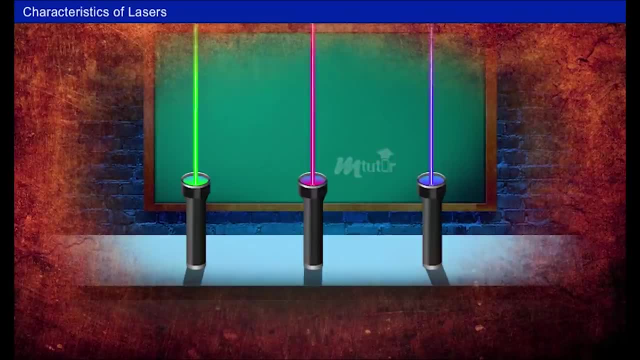 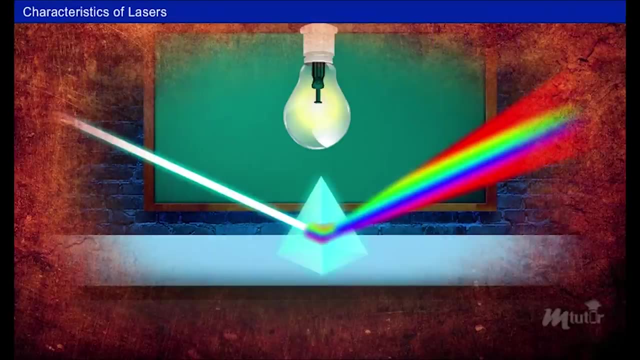 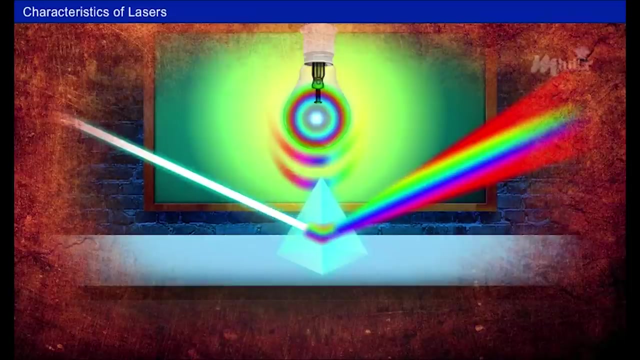 Laser lights are highly monochromatic. It means the laser beam is made up of a single color or a single wavelength. In contrast, the ordinary white light from an incandescent light bulb is a combination of many colors or wavelengths and is certainly not monochromatic.